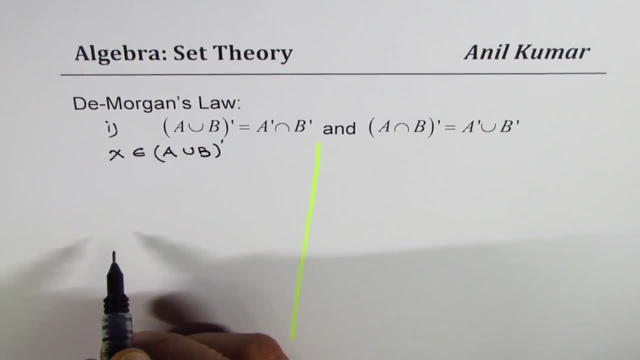 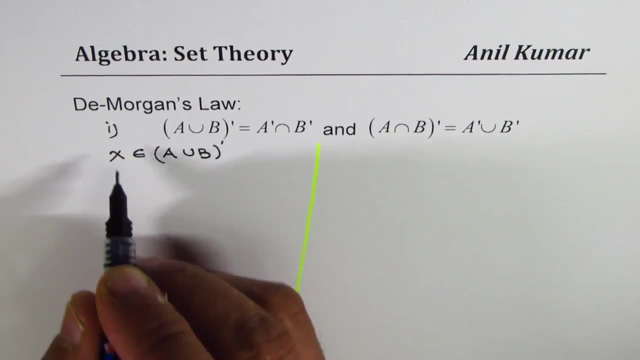 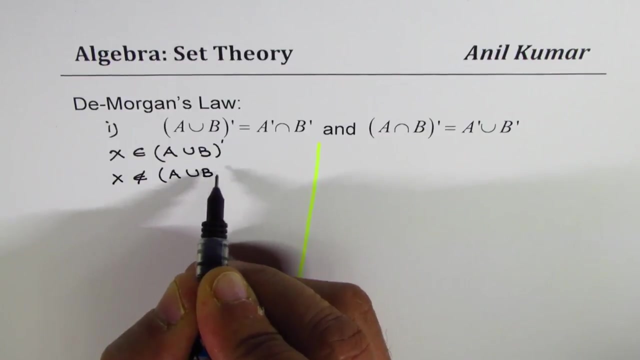 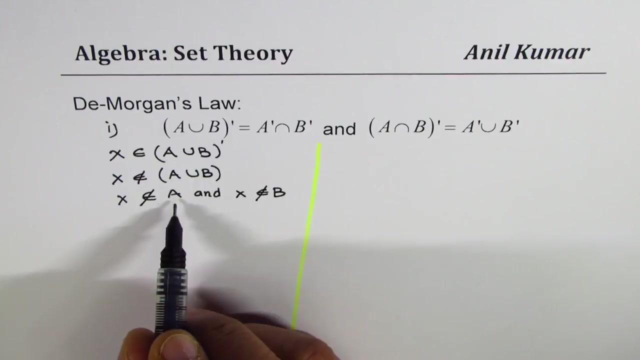 complement of A union B, right. So if it belongs to complement of A union B, that means that X does not belong to A union B, correct? or it means that X does not belong to A and X does not belong to B, right? So X does not belong to A and X does not. 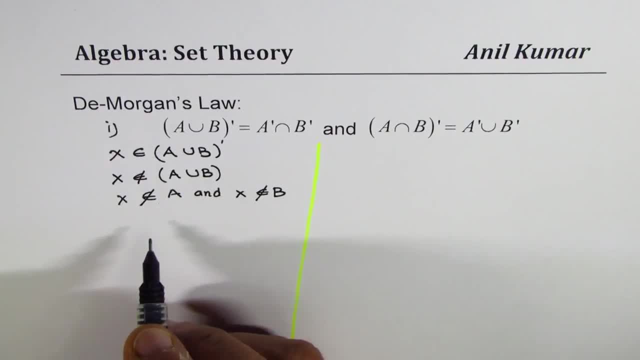 belong to A- B. that means their intersection, right. ok, That also means that X belongs to. I mean, I have to write X. X belongs to complement of A. if it does not belongs to A, it belongs to complement of A and X belongs to complement of B. With that we can say that X belongs. 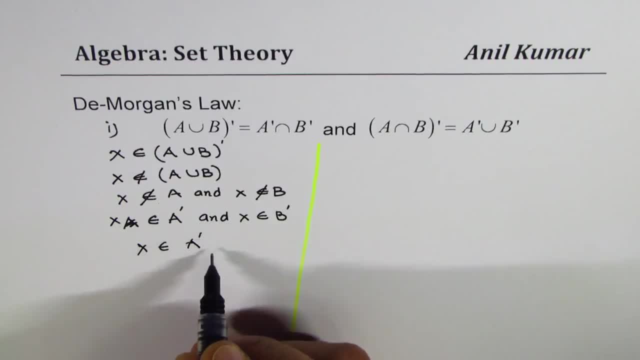 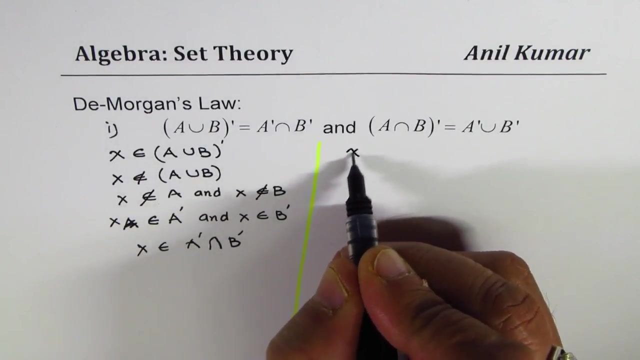 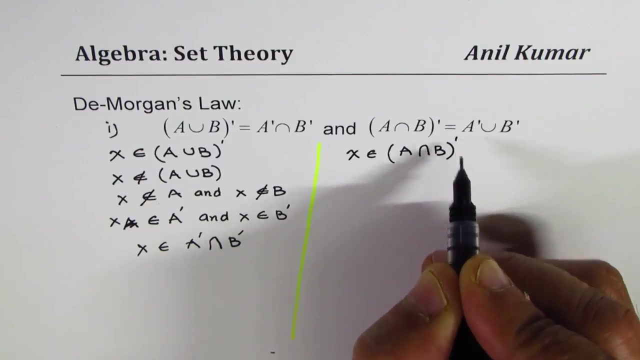 to A complement And means intersection of B, correct. so that is how you can prove it. Now similar guidelines can be used to prove the second part. so let us begin by saying that X belongs to A intersection B complement, right? So that means that X does not belong. 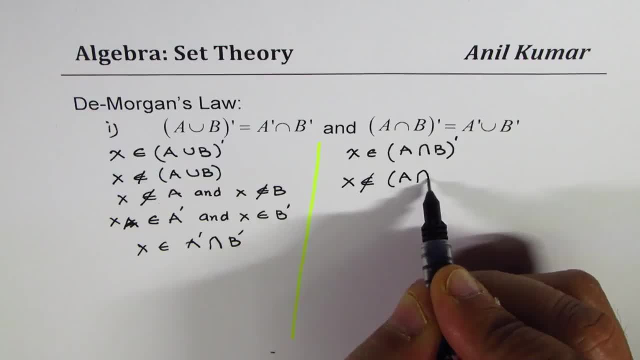 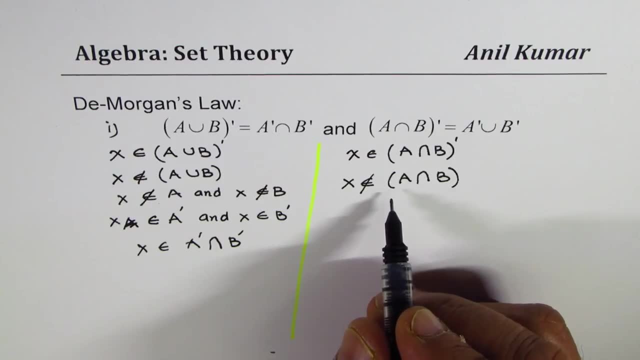 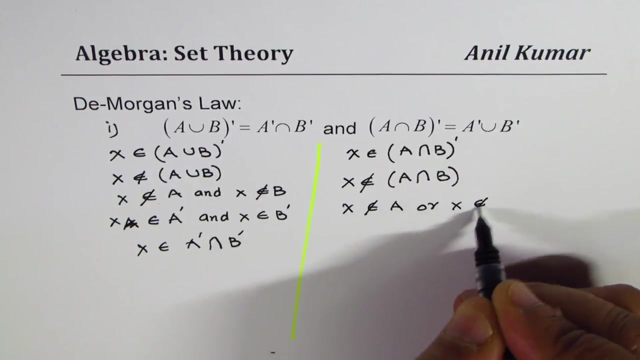 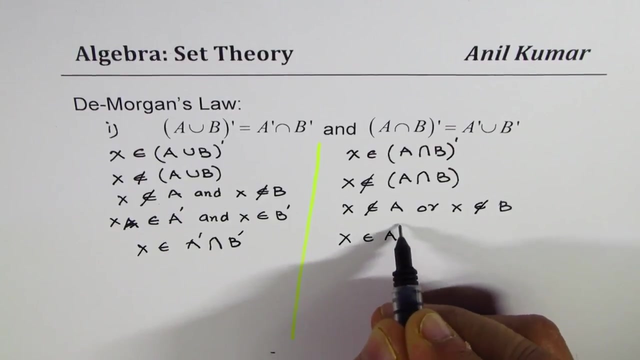 to intersection of a and b. right, so it does not belong to the intersection of a or b. so that really means that x does not belong to a or x does not belong to- i mean, does not belong to b. if it does not belong to a, then x should belong to complement of a or x should belong. 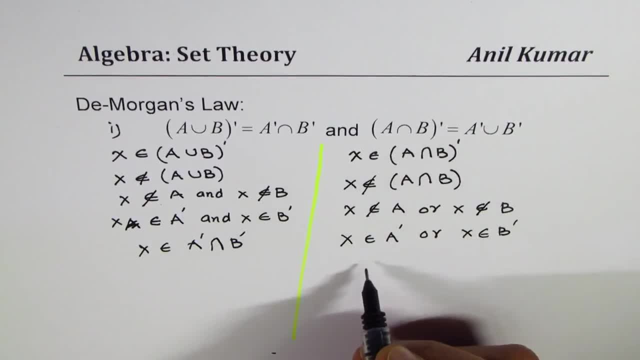 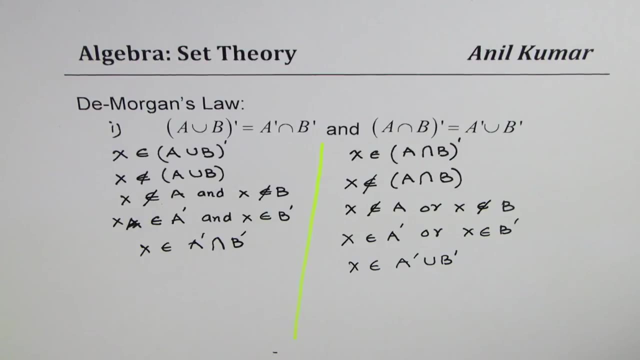 to complement of b and that gives us x belongs to a complement union, b complement right. so that becomes a proof for de morgan's law and we can use it in proving many of the properties in set theory. amal kumar, and i hope that helps. thank you and all the best.